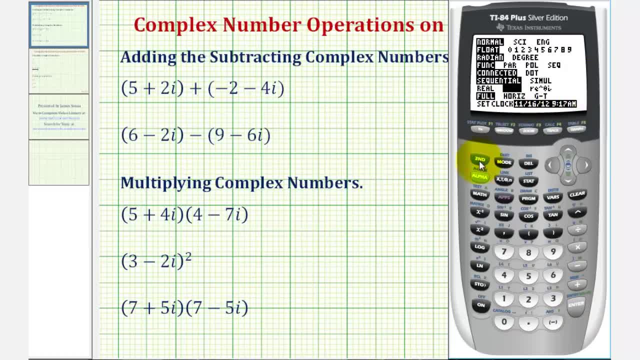 complex mode. So now we'll go back to the home screen by pressing second mode, and now we can perform complex number operations. So we'll first find the sum of these two complex numbers and the difference of these two complex numbers. So we'll have open parenthesis. 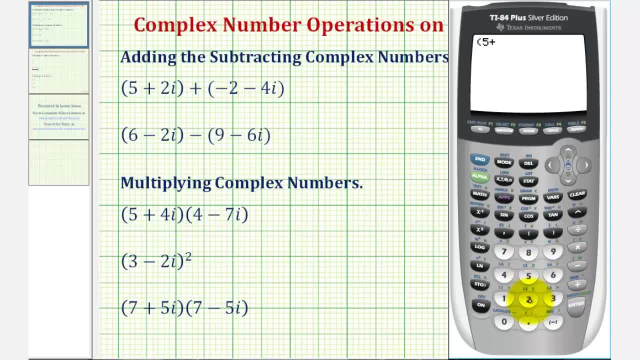 five, six, seven, eight, nine, five plus two i, So two, and then the i is second decimal point. So second decimal point brings up i, the imaginary unit, close parenthesis plus open parenthesis, negative two minus four i. Again, the i is second decimal point, close parenthesis. 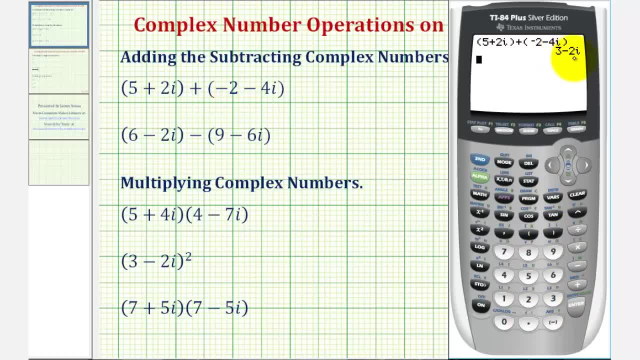 and enter. So our sum is three minus two, i. Let's also find the difference. So we have six minus two, i closed parenthesis. Mamus nine minus six, i closed parenthesis. So the difference of these two complex numbers is negative. three plus four, i. So again the sum is three. 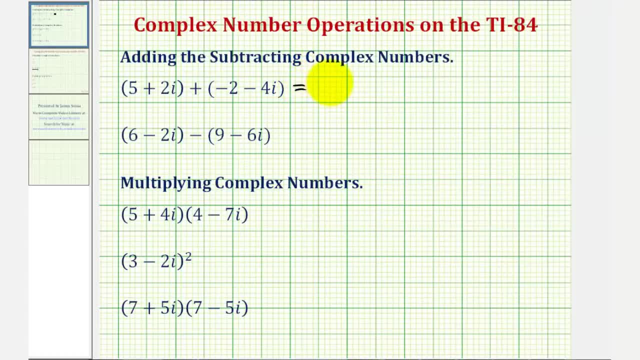 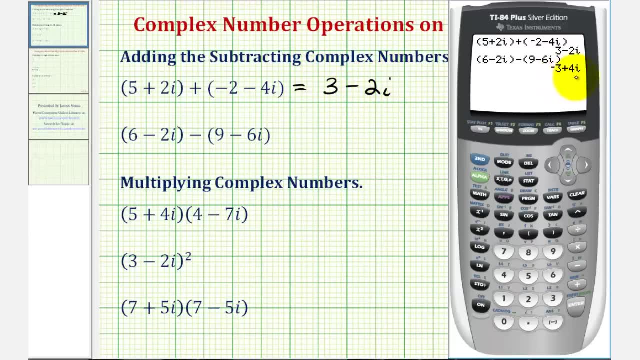 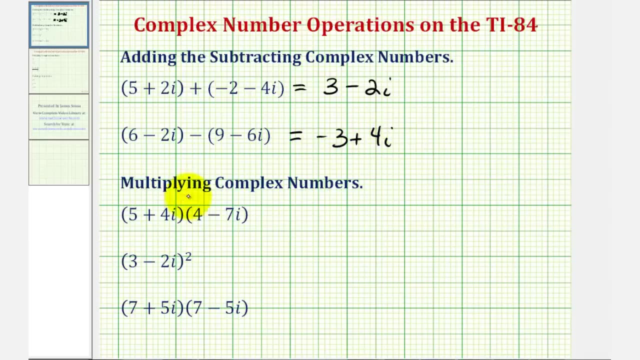 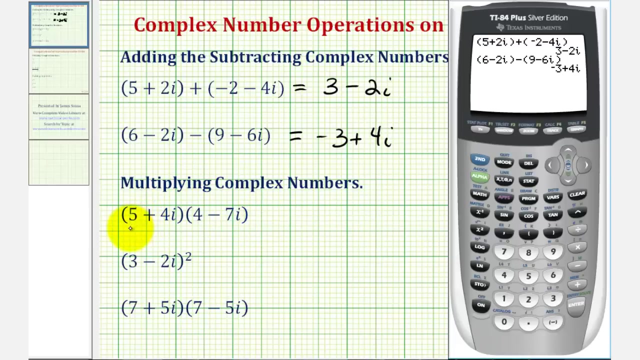 minus two i and the difference is negative: 3 plus 4i. Now we'll look at products of complex numbers. So in our first example we have the complex number 5 plus 4i times the complex number 4 minus 7i and enter and the product will be 48 minus 19i. 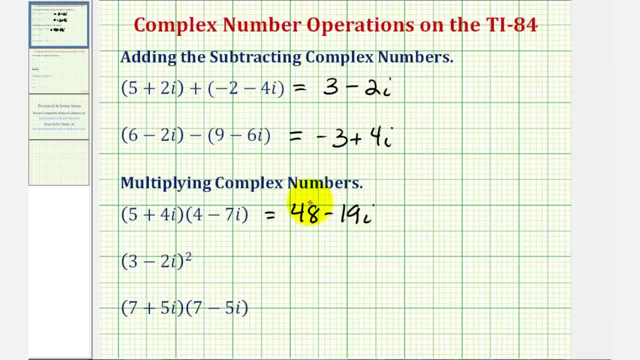 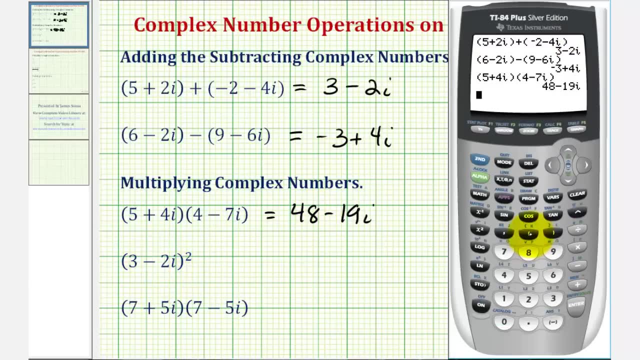 So, as you can see, once the graphing count is in complex mode, we really just need to type in what we see. Next we're squaring the complex number 3 minus 2i, so, open parenthesis, 3 minus 2i. 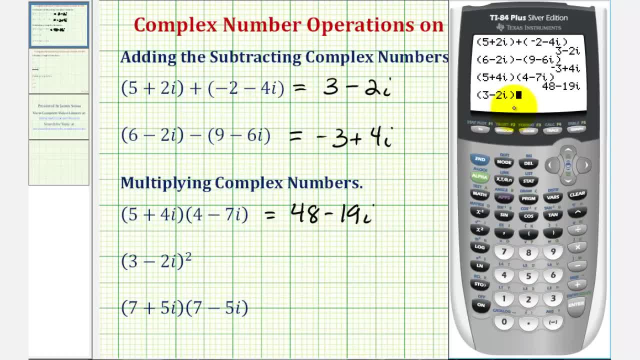 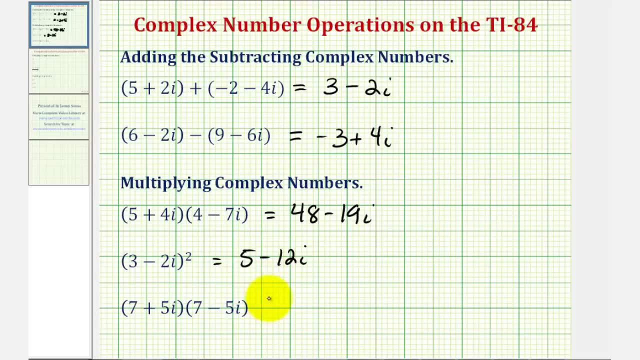 Again, i is second decimal point, close parenthesis. then to square this, we'll press x squared and then enter. So the square of 3 minus 2i is equal to 5 minus 12i. Now looking at our last example, 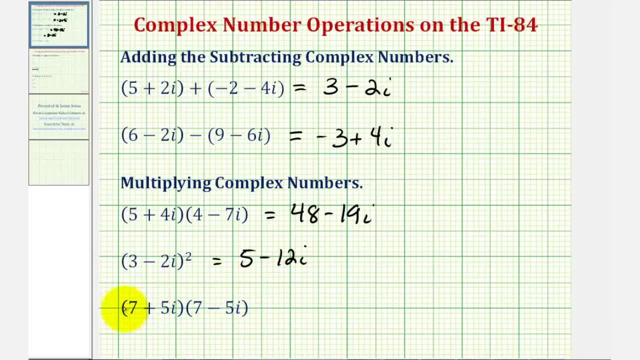 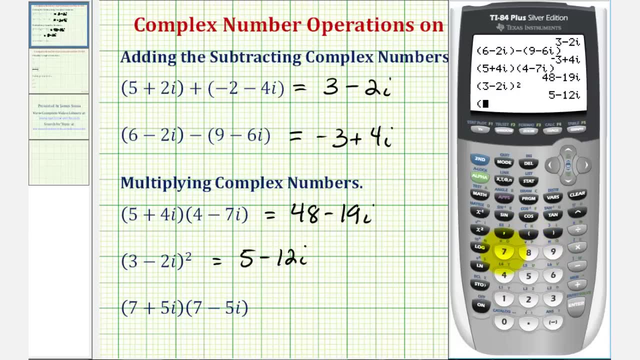 of a product. notice how these are complex conjugates, so this product will be a real number. Let's go ahead and verify that. We have 7 plus 5i times 7 minus 5i, And the product is equal to 74.. 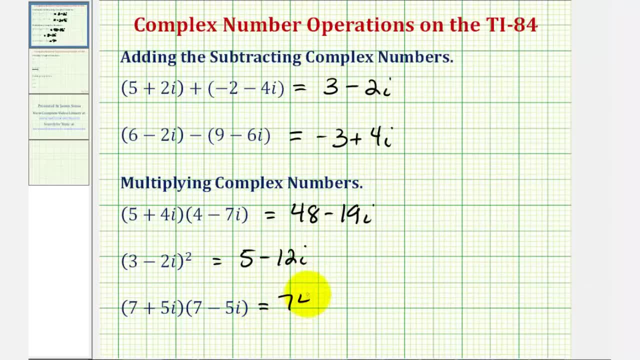 So these really aren't that difficult to do by hand- and I do have videos that explain how to do all these by hand, but it is nice to be able to check our answers on the graphing calculator. Now let's take a look at quotients and raising i to various powers. 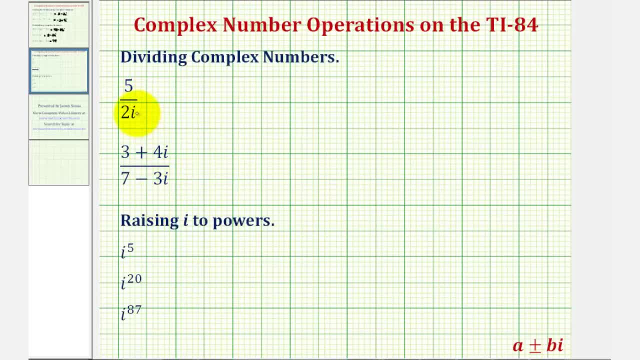 Looking at our quotients, notice how, for a complex number, we're not allowed to have i in the denominator. normally what we do is multiply the numerator and denominator by the conjugate of the denominator. But again, for these examples, we'll perform this division on the graphing calculator. 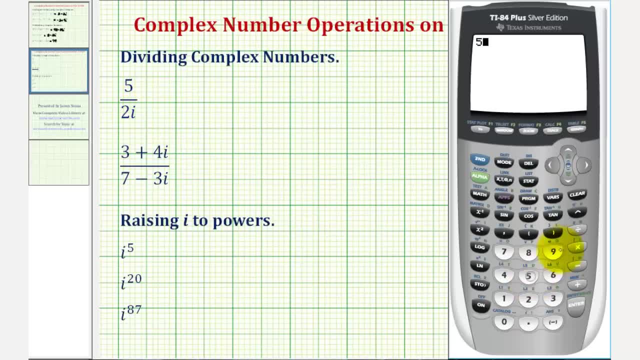 So we have 5 divided by 2i. so we're going to put 2i in parenthesis. so 2. second decimal point, close parenthesis- enter. Now we want this back in fraction form, so I'm going to go ahead and press math: enter: enter. 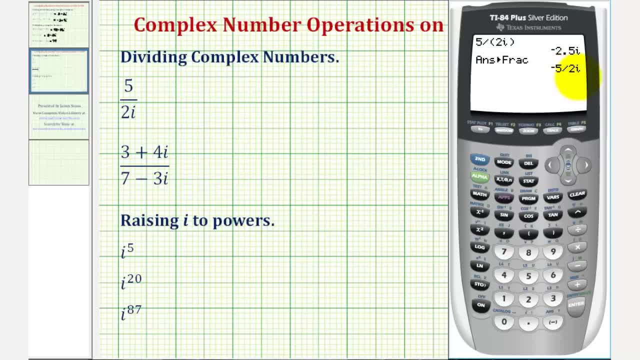 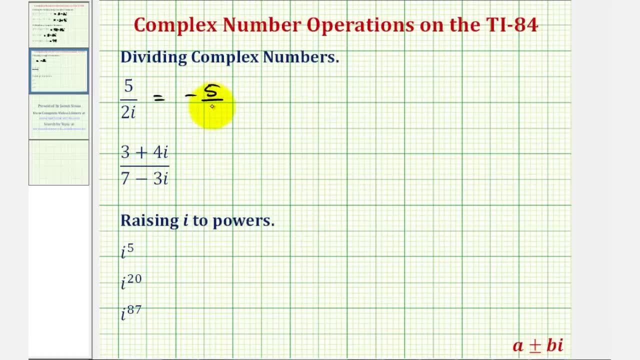 Now we need to be careful here. This is negative 5.5. I not negative 5 divided by 2i. So this is equal to negative 5.5i or, if we want, we could write this as negative 5i over 2.. 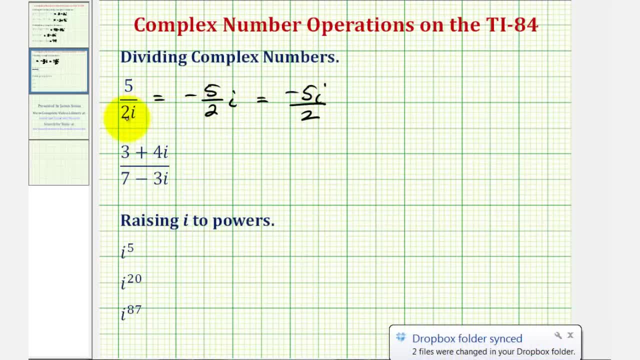 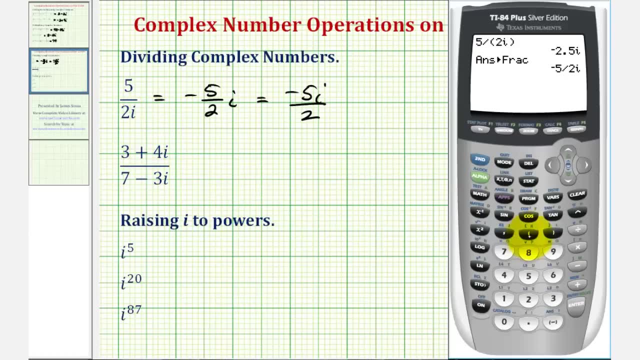 The i is not in the denominator because we know that's what we started with. we're not allowed to have i in the denominator. Now let's take a look at our second example of division. We have the complex number 3 plus 4i. 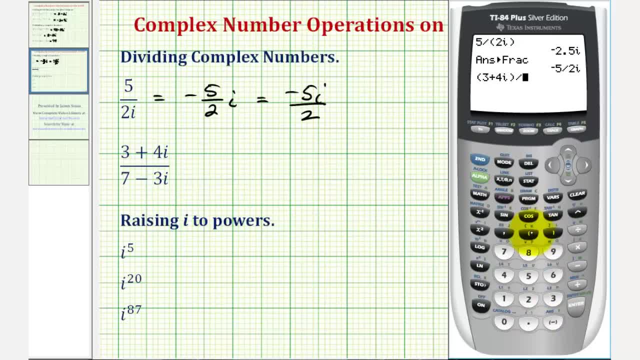 Divided by the complex number 7 minus 3i. And these parenthesis are necessary to indicate which complex number is in the numerator and which is in the denominator. So press enter. Notice how this is messy. so we'll convert this back to a fraction by pressing math enter enter. 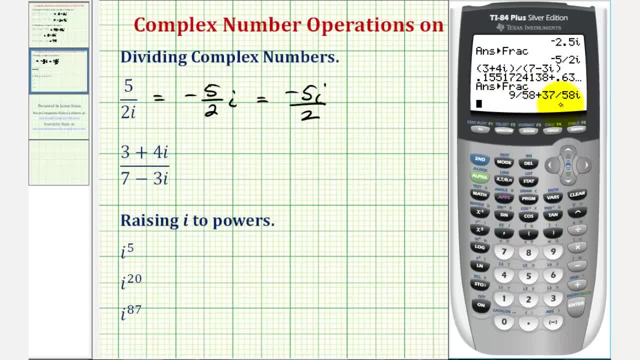 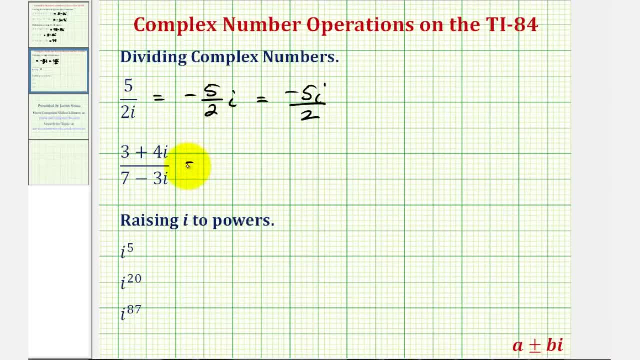 So we have 9 58ths plus 3i. Notice how the calculator is giving us the complex number in standard form, with a form a plus or minus bi. So we have 9 58ths plus 37 58ths i. 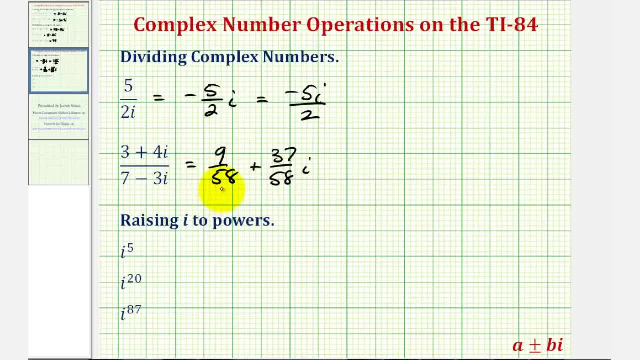 Notice how the calculator is giving us the complex number in standard form with a form, a plus or minus bi, but a lot of times, when doing this by hand, we write this as a single fraction. this is equivalent to 9 plus 37.. 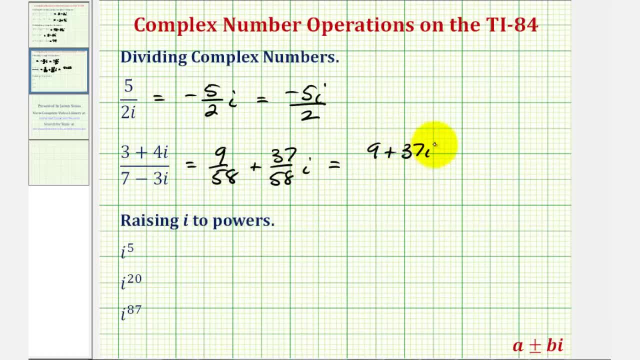 thirty-seven, i all over fifty-eight. Again, it's important to recognize that the i here is not in the denominator. Now for the last three examples. we're going to raise i to various powers, and as long as the power isn't too large, the calculator does fine with it. but we'll notice something strange on this last example. 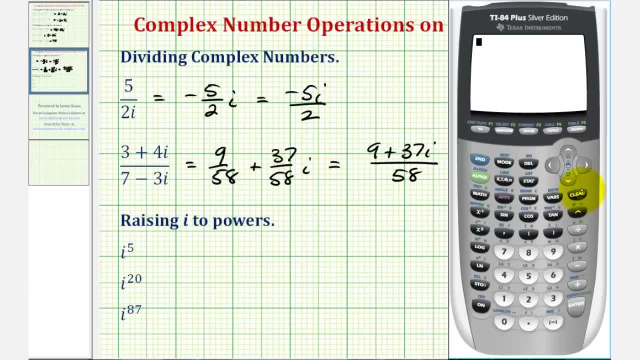 So we have second decimal point for i raised to the fifth power, which is equal to i. Next we'll find i raised to the twentieth power. So second decimal point and then exponent twenty is equal to positive one. So let's go ahead and write these two down. So i to the fifth is equal to. 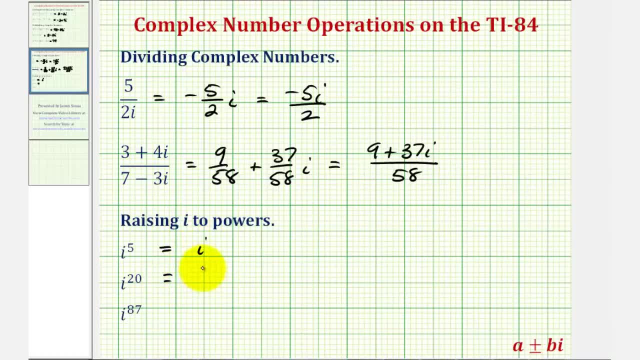 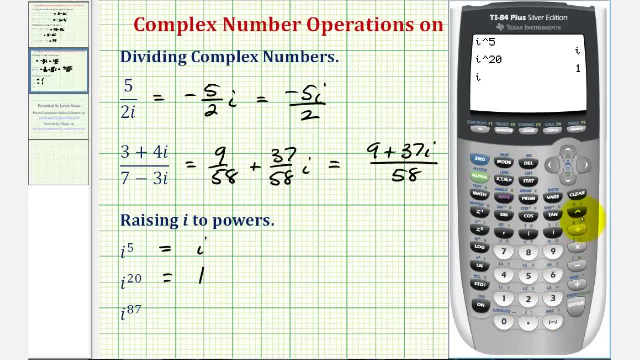 i and i to the twentieth is equal to positive one. And now for this last example. we'll have second i raised to the power of eighty-seven and enter. Now notice how the real part of the complex number, or a, is equal to three point seven times ten to the negative twelfth. 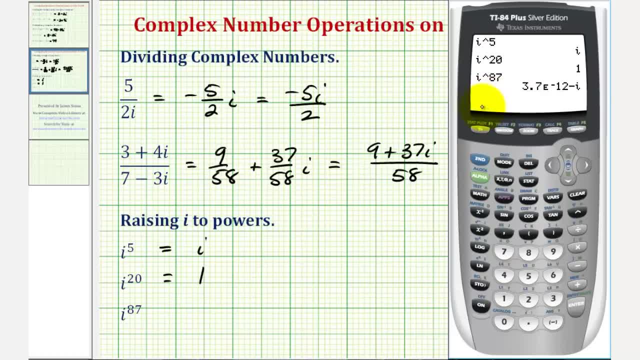 This is really not the value of a. The calculator is having a problem determining a. Notice how this would be a very, very small number. and it's actually zero because we know we raise i to a power, it's either i negative, i one or negative one, So we can disregard this first part. 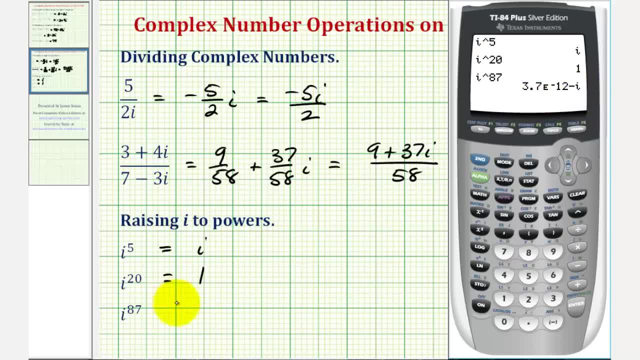 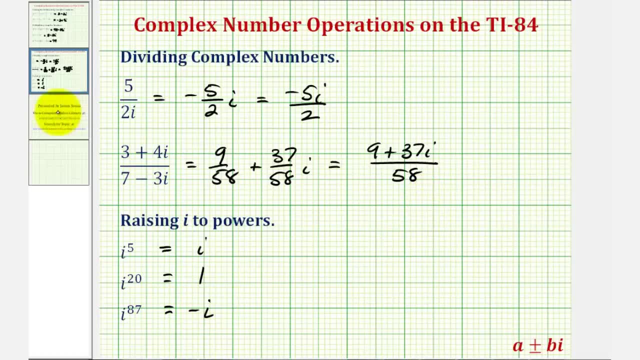 and i to the eighty-seventh. power is equal to negative. i Okay. I hope you found these examples helpful.